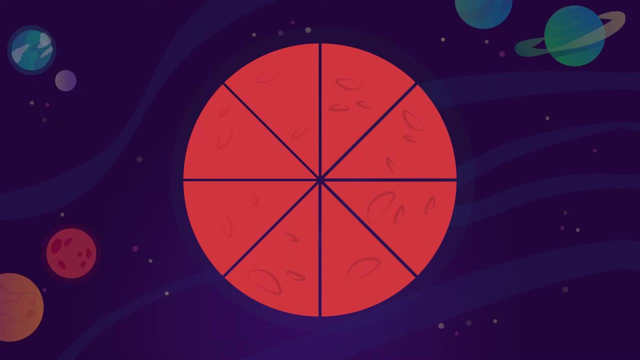 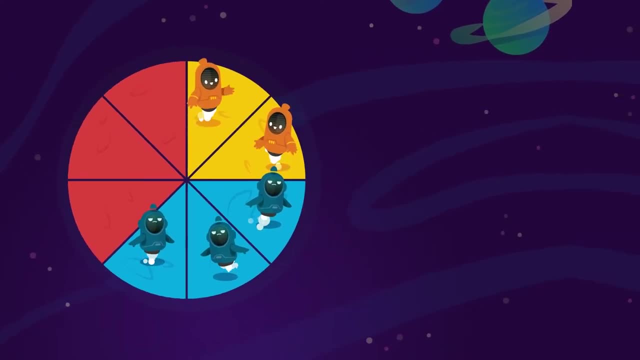 Two-eighths of the planet are occupied by friendly aliens and the remaining three-eighths by grumpy aliens. Can you guess what fraction each alien is? The ones for each alien: two-eighths of the alien. three-eighths of the planet. What fraction would represent this number as an way of adding? 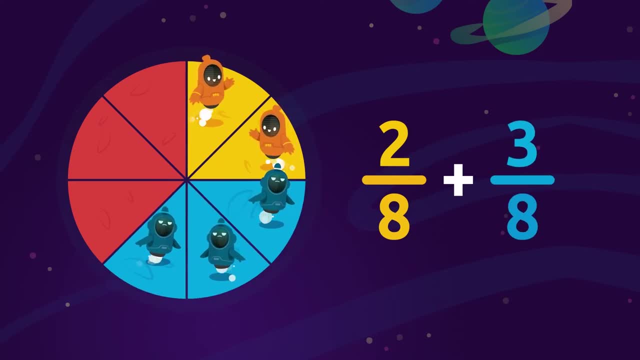 more fractions. and how do we multiply all the aliens on the planet? And outright, How possessive is this number? Let's think about it. How can we multiply a fraction by saying Nam's name, due to our Remember how to do this math operation. 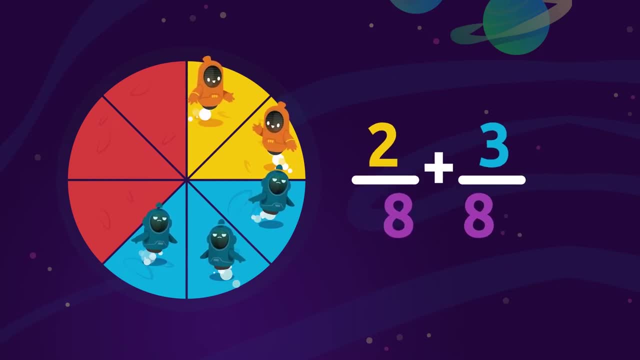 Remember that the result would have to be the same denominator. In this case it would be the number 8.. And now to calculate the numerator, we'll add the numerators 2 and 3, which equals 5.. The result will be that 5 eighths of the land are occupied by aliens. 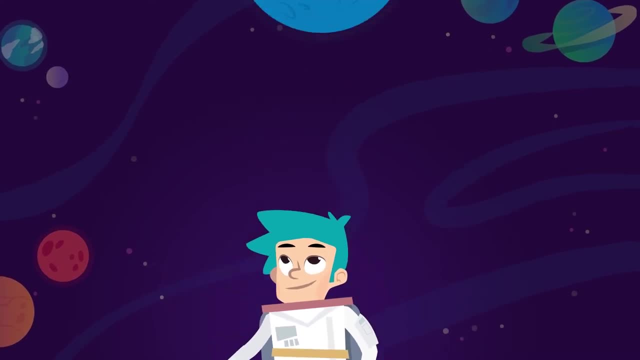 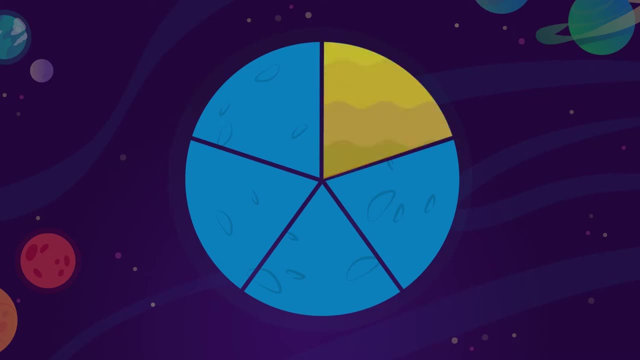 Will you help me figure out something else, Learnython? our neighboring planet is divided into 5 equal parts. There is yellow water on 1 fifth of the planet, purple water on 3 fifths of the planet and volcanic soil on 1 fifth of the planet. 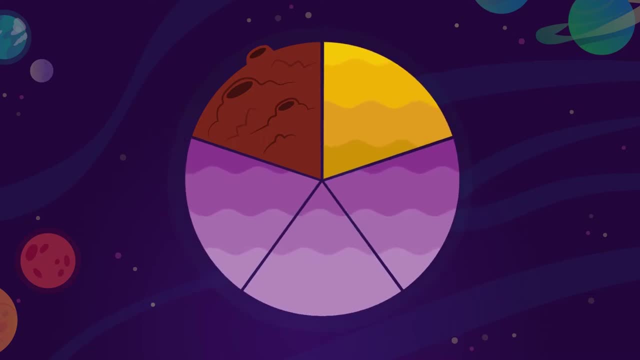 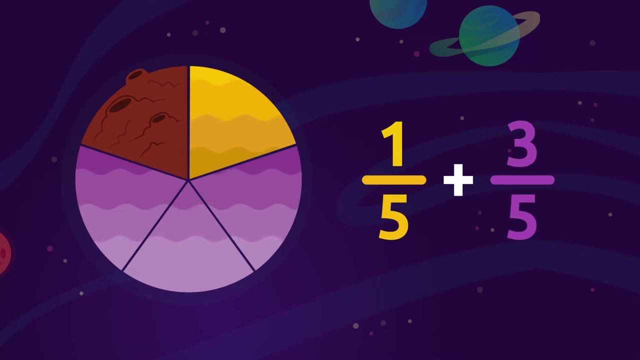 How much of the land on planet Learnython is covered with water. To find out, we'll need to add the fractions 1 over 5 plus 3 over 5.. First in the result we'll leave the common denominator and then we'll add the. 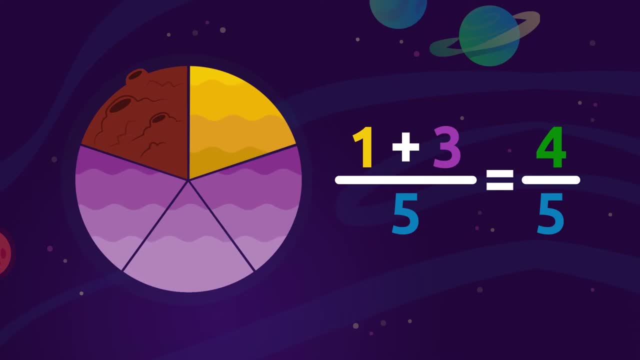 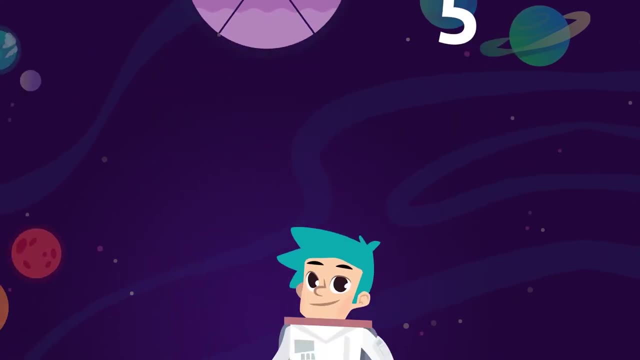 numerators 1 plus 3, which equals 4.. The result will be that 4 fifths of the land of the planet are covered with water. Thank you for helping me. Now you know how to add fractions with the same denominator. 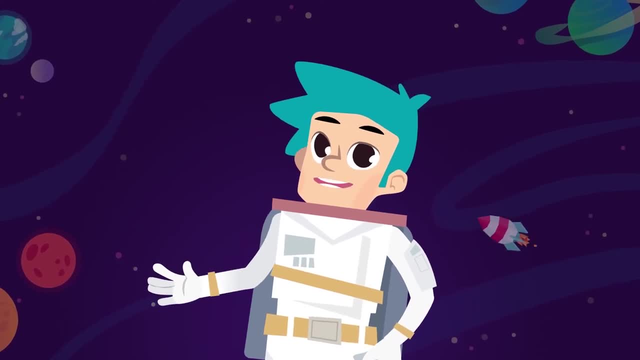 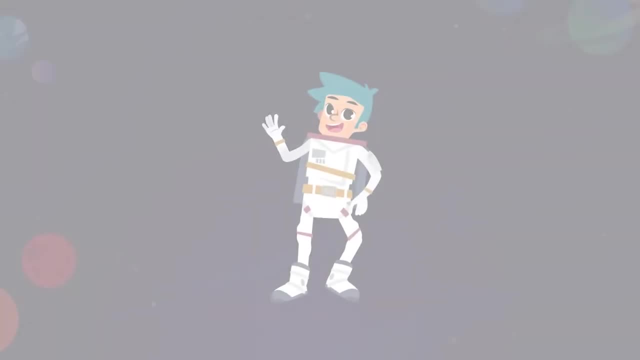 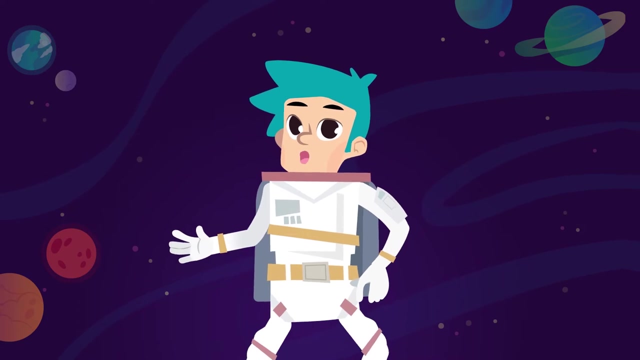 Little by little, you're going to become math experts. Keep up the good work. See you around. Hello again, math friends, We're going to continue learning about fractions. Today, we're going to learn how to subtract fractions with the same denominator. 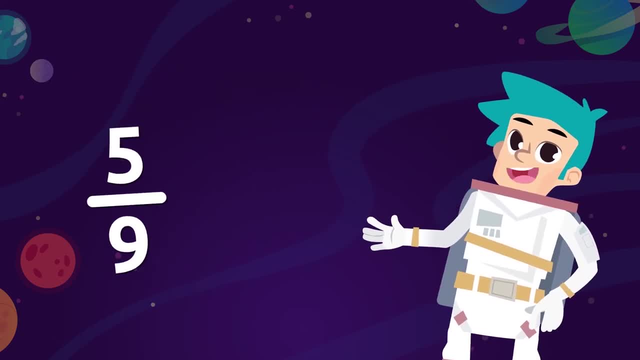 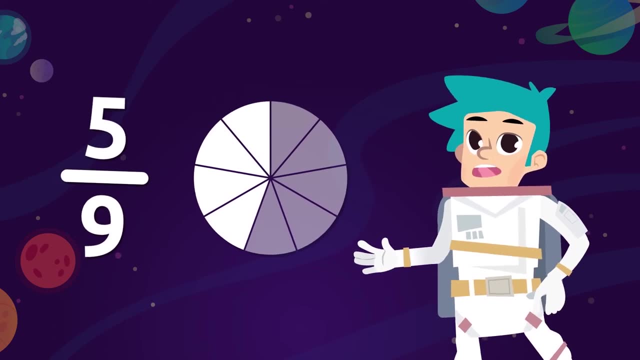 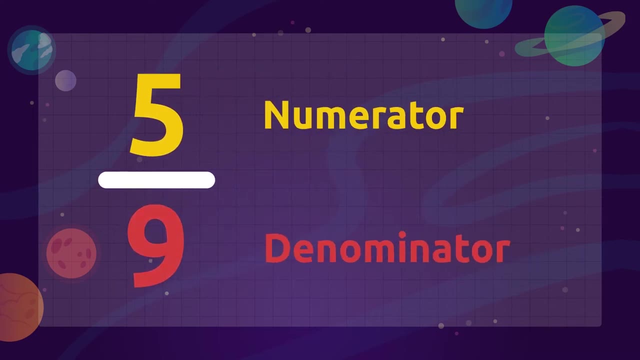 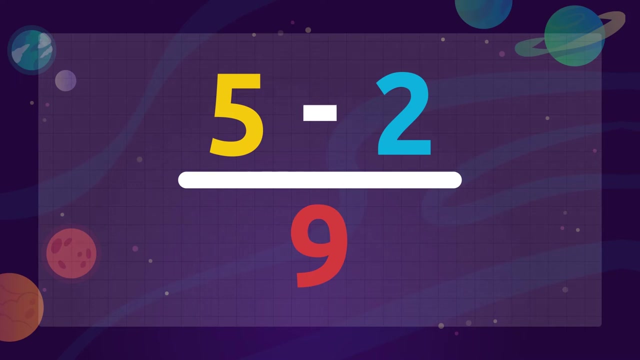 Do you remember what a fraction is? A fraction is a number which indicates the division of a whole number in equal parts. First let's remember which are the parts of a fraction. This is the numerator and this number is the denominator To subtract fractions with the same denominator. we leave the common denominator and only subtract. 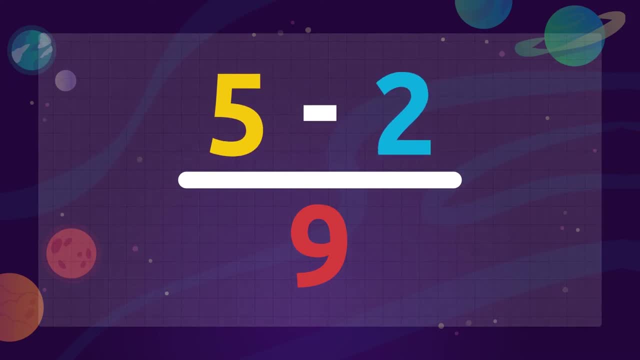 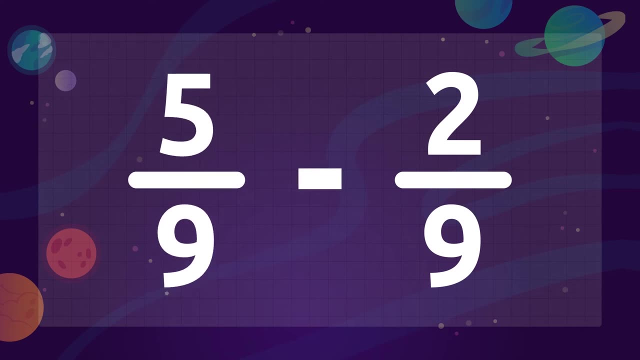 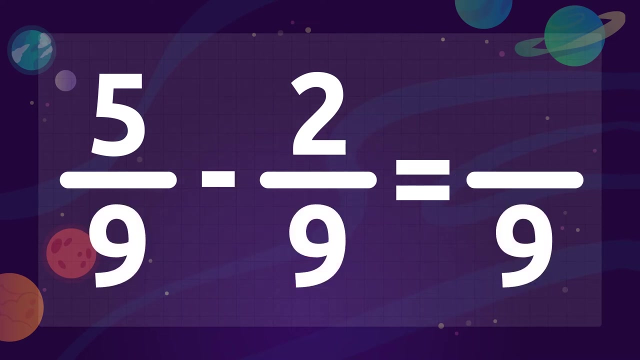 the numerators. It's very simple. Let's see an example. We need to solve this math problem: 5 ninths minus 2 ninths, The denominator stays the same. In this case it's the number. Now we subtract the numerators. 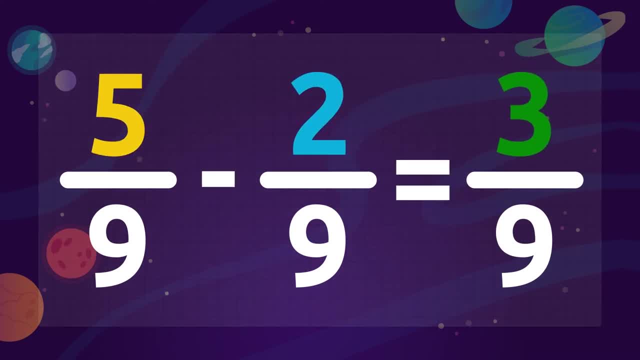 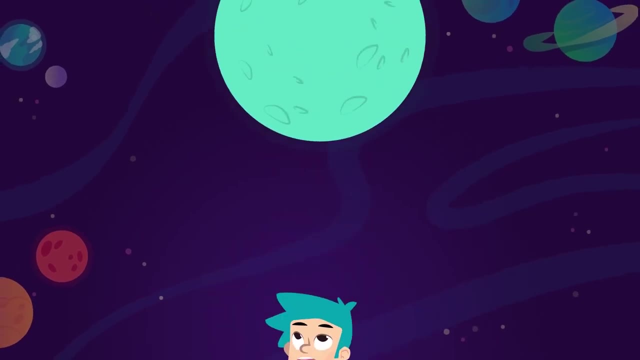 That is 5 minus 2, which equals 3, which will be the numerator in the answer. The result of this math problem will be 3 ninths. Are you up for a challenge to practice a bit more In the Smile and Learn universe? there's a planet called Smileython. 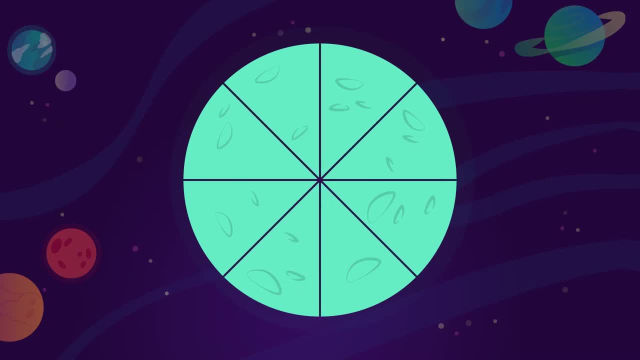 The planet is divided into 8 parts. It's called Smileython. It has 8 equal parts. In 6 of these 8 fields they grow apple trees and lemon trees. If 4 of the 8 fields are planted with lemon trees, how many fields are planted with apple? 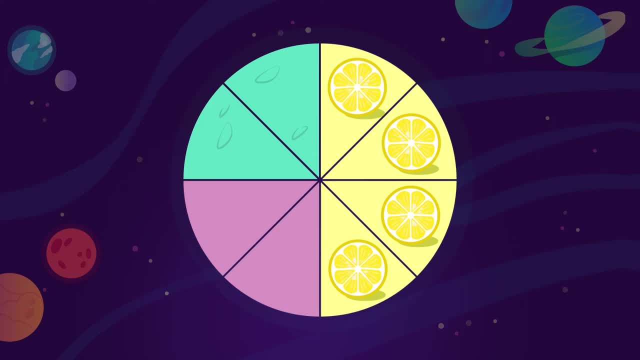 trees. To find out, we'll have to subtract fractions. We need to subtract the total number of fields planted with fruit trees from the number of fields planted with lemon trees To find out how many apple tree fields there are, Meaning 6 eighths minus 4 eighths. 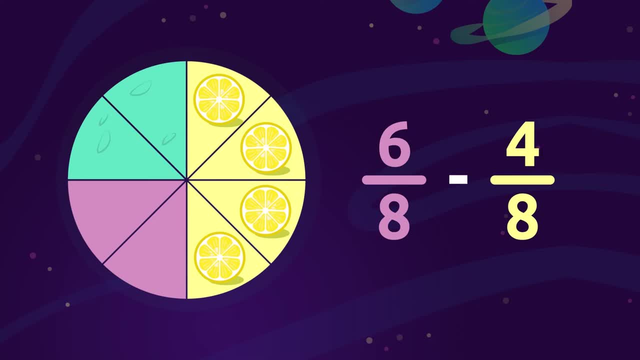 Do you remember how to do this math operation? Remember that we should put the same denominator in our answer, In this case number 8.. Now to calculate the numerator, we subtract the numerator's 6 minus 4, which equals 2.. 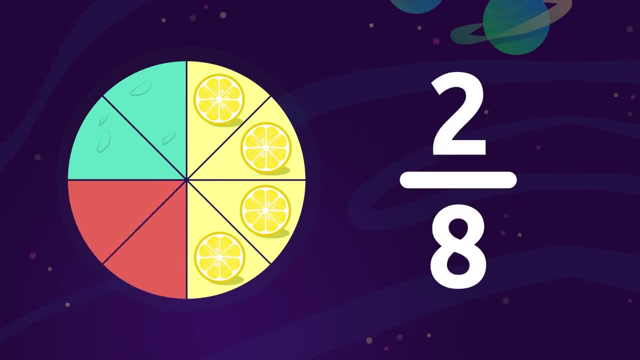 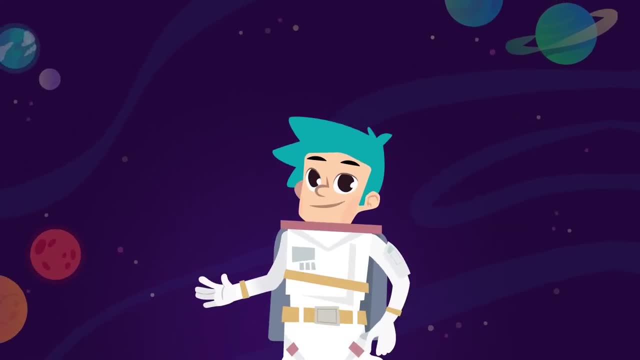 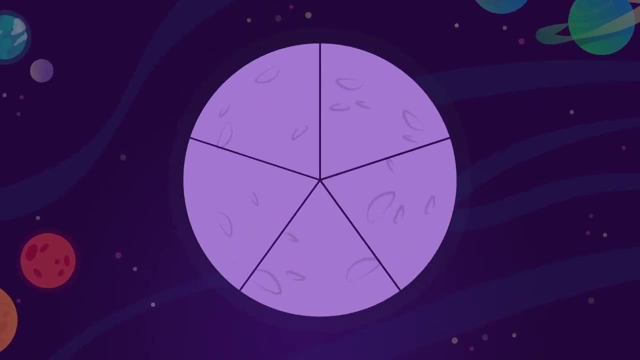 2. The result is that 2 of the 8 fields are planted with apple trees. That is 2 eighths. Will you help me figure out something else? Planet Learntern is divided into 5 equal parts. On this planet there are wooded areas and areas with houses. 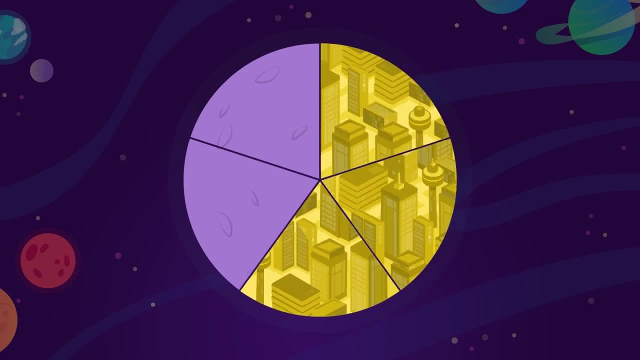 If they built houses on 3 of Learntern's fields, how many parts of the planet are cut? How many parts of the planet are covered with woods? To find the solution, we'll need to subtract the fractions 5 fifths minus 3 fifths. 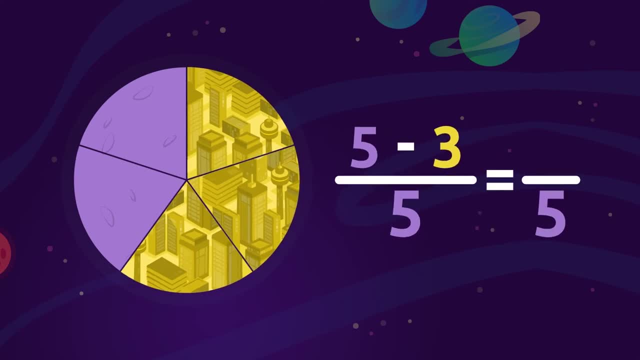 To work out the answer, first we leave the same denominator, In this case it's number 5.- And then we subtract the numerators, In this case 5 minus 3, which equals 2.. 2., 2.. 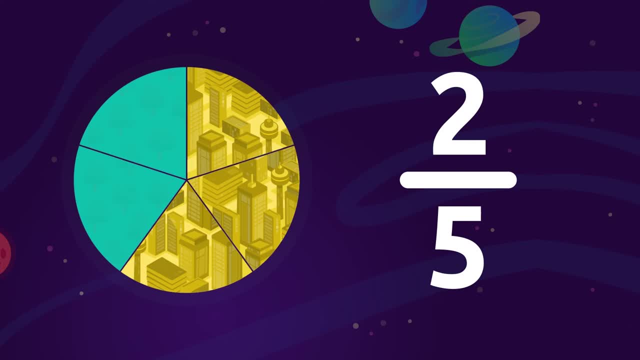 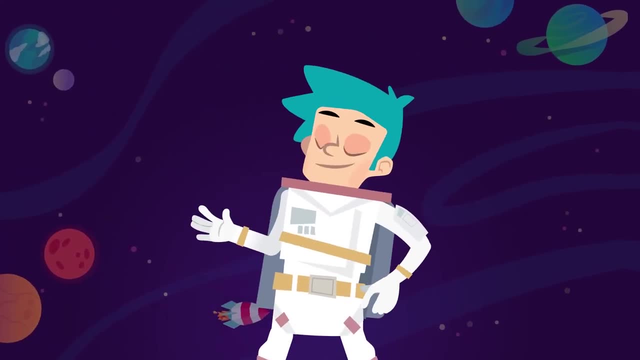 It's 7. 6 times 3.. 0., 1., 9., 6., 4., 5., 5., 2., 3., 6., 7., 6., 9. 8.. 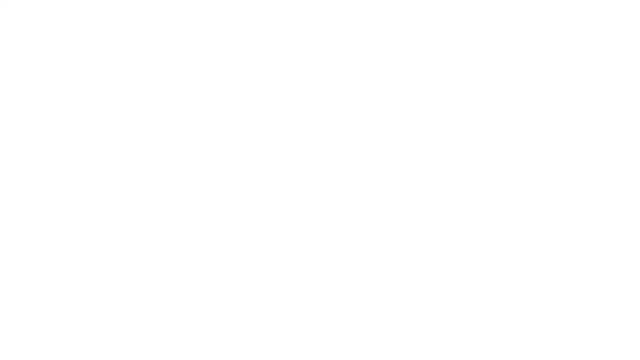 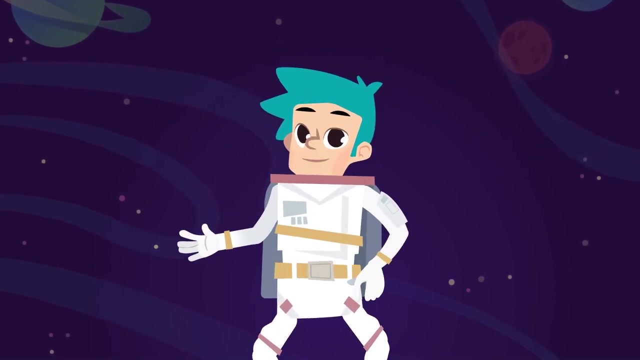 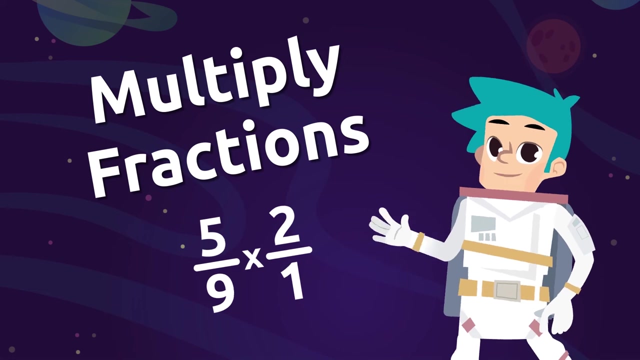 7., 12. 5., 4., 1., 6., 1., 2., 2., 7., 5., 1., 1., 3.. multiply fractions. First let's recap the parts of a fraction. 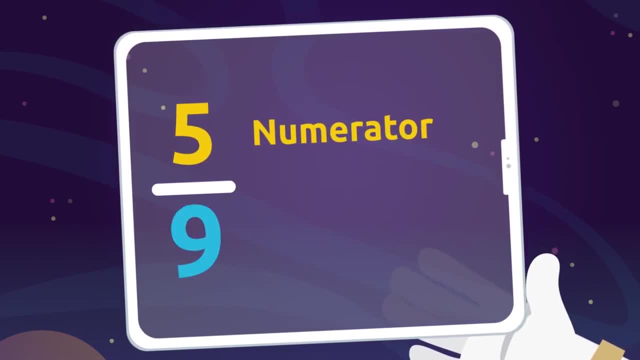 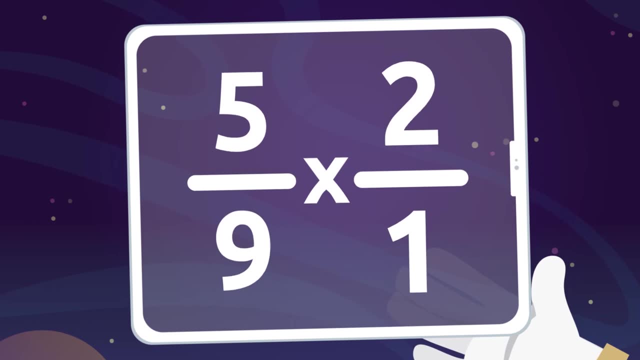 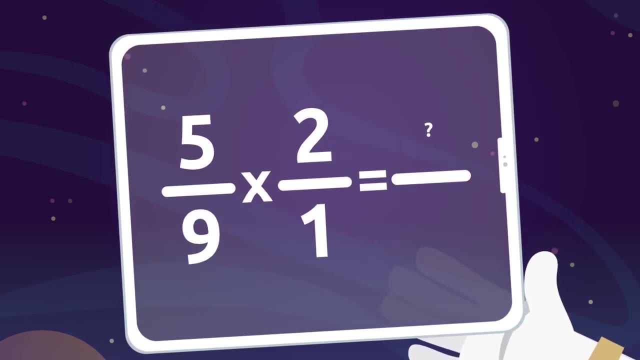 The top number is the numerator and the bottom number is the denominator. Now we're ready to start. Do you know how to multiply fractions? It's really easy. pay close attention. To find the numerator, we multiply the numerators. and to find the denominator, multiply the denominators. 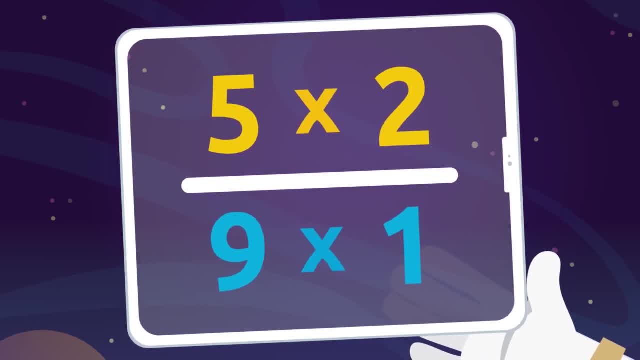 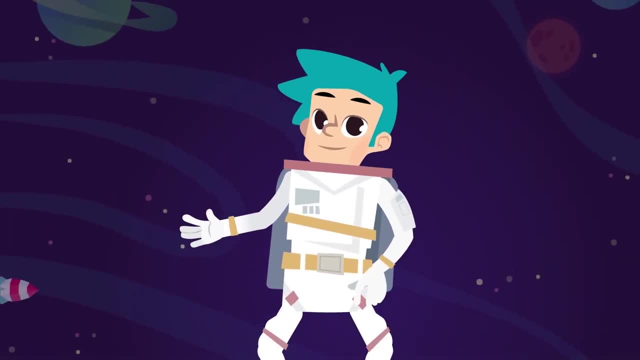 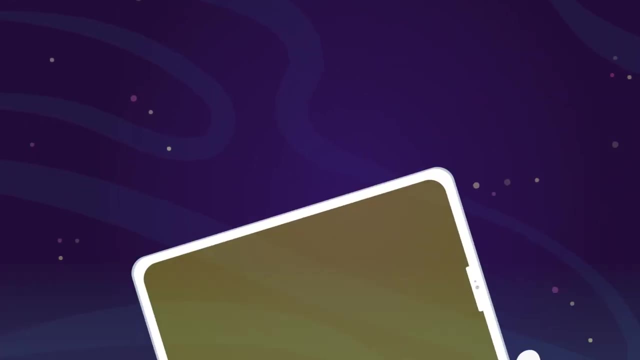 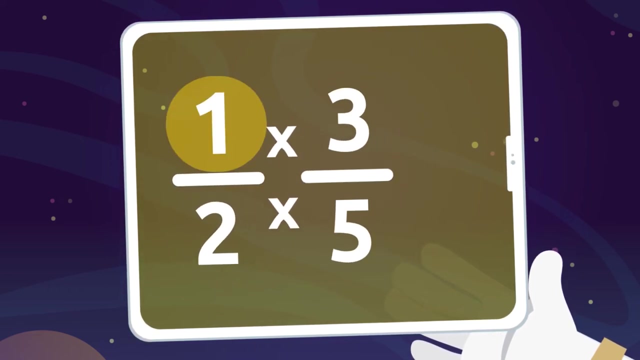 This means that to multiply fractions, we multiply the two numerators together and the two denominators together. Easy, right told you. Let's look at an example. We need to multiply 1- half by 3- fifths. To do that, we're going to multiply the numerators 1 by 3, which equals 3. 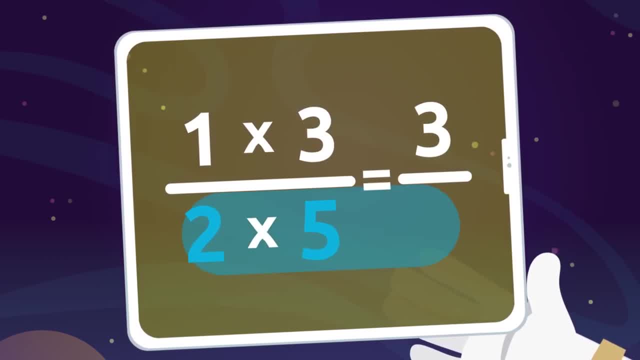 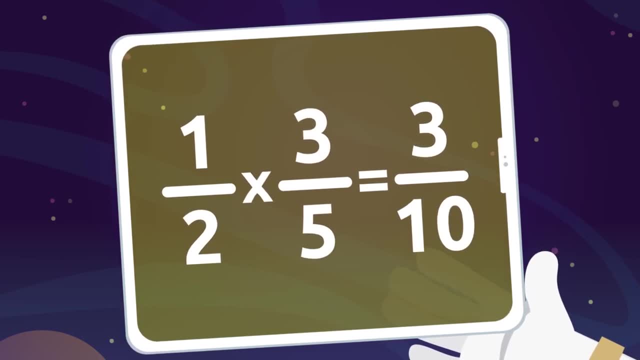 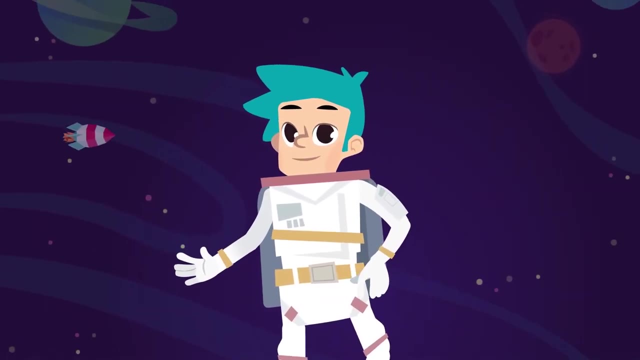 And then we're going to multiply the denominators 2 by 5, which equals 10. So 1 half multiplied by 3 fifths equals 3 tenths. Well done, Did you understand that? shall we look at another example? let's see if you can solve this operation. 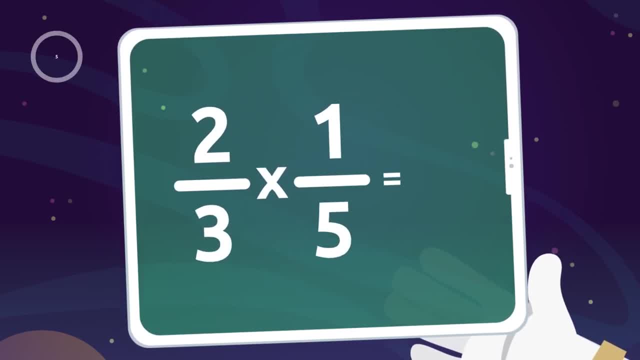 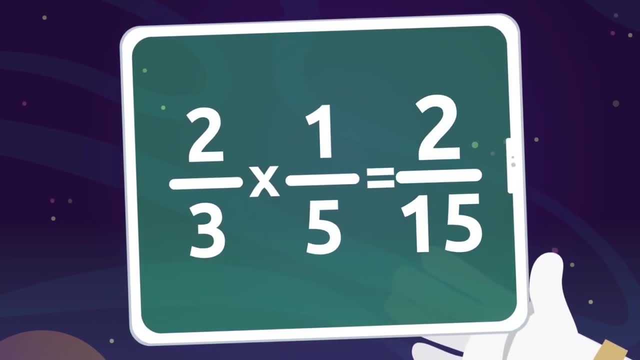 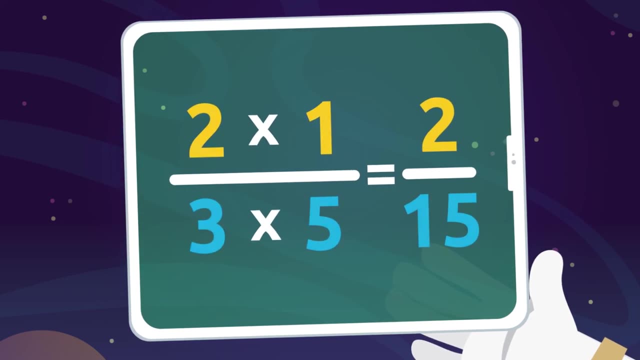 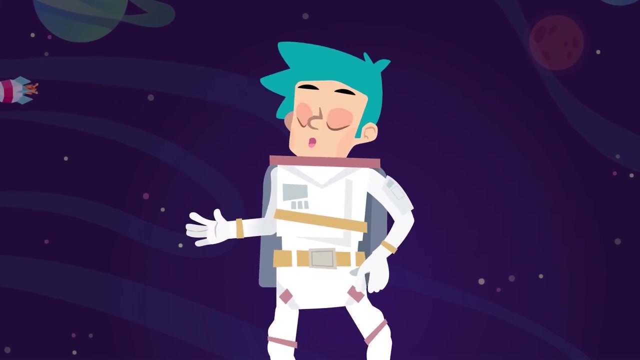 2 thirds multiplied by 1 fifth equal 2 fifths. 2 by 1 equals 2. and 3 by 5 equals 15.. Did you get that right? amazing Congratulations. now you know how to multiply fractions. You're a real expert. See you on the next video. 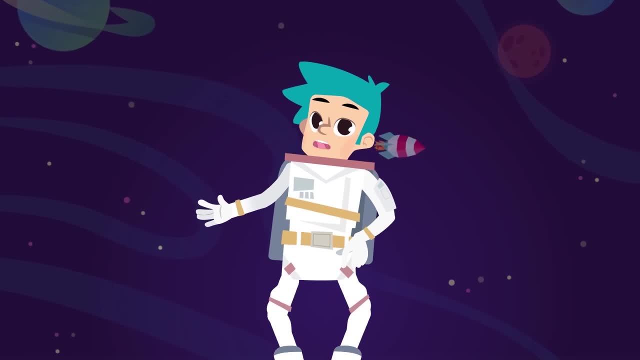 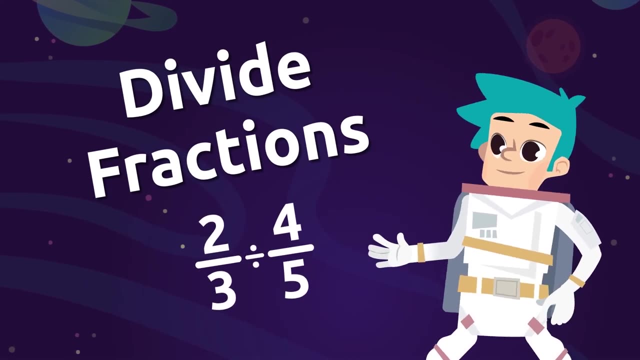 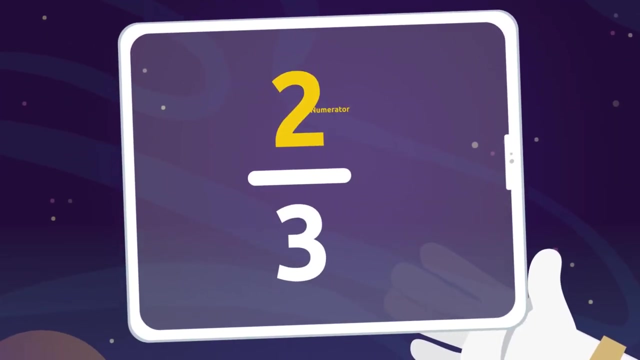 Hello again, friends, We continue practicing operations with fractions. today We're going to learn how to divide fractions. First, let's recap quickly the parts of a fraction: The top number is the numerator and the bottom number is the denominator. now we're ready to start. 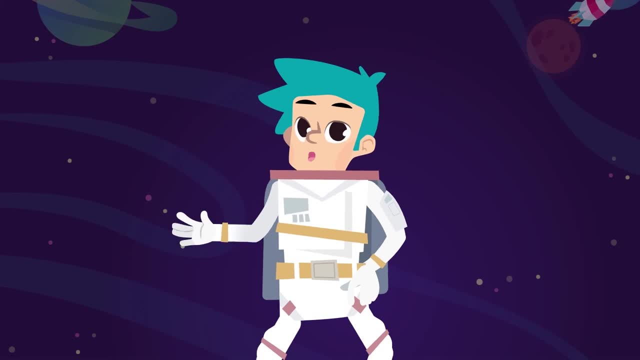 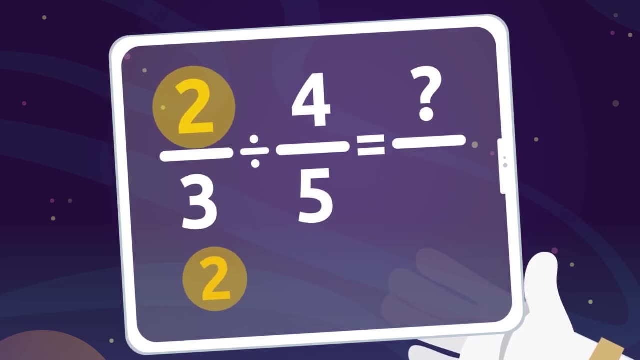 Dividing fractions is fun. Do you want to know how it's done when we divide fractions? to Find the numerator? we should multiply the numerator of the first fraction by the denominator of the second fraction. To find the denominator, we multiply the denominator of the first fraction by the numerator of the second fraction. 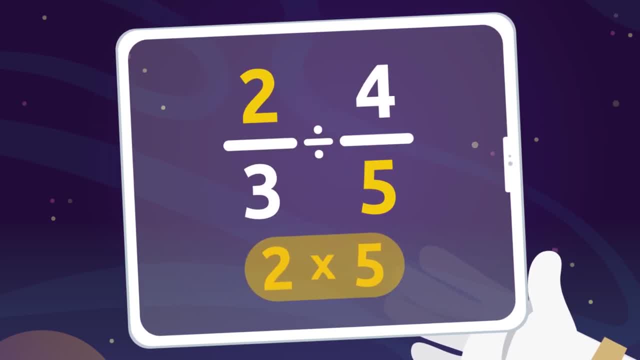 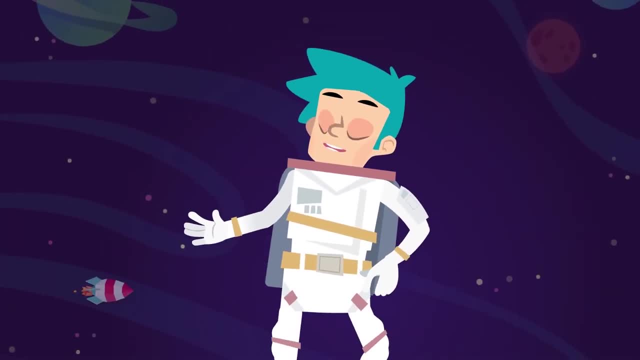 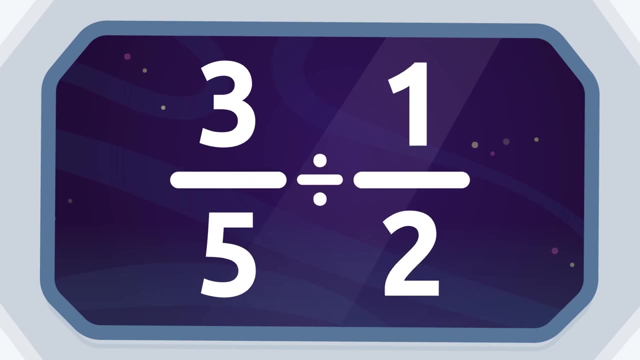 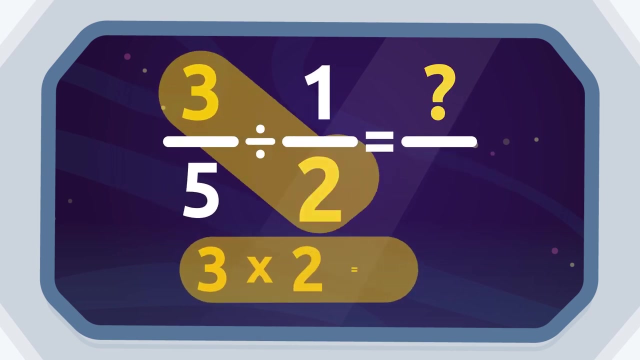 This means that to divide fractions, we cross, multiply them. Did you understand how it's done? let's look at the next example. We need to divide 3 fifths by 1 half To find the numerator of the product. we multiply the numerator of the first fraction by the denominator of the second fraction. 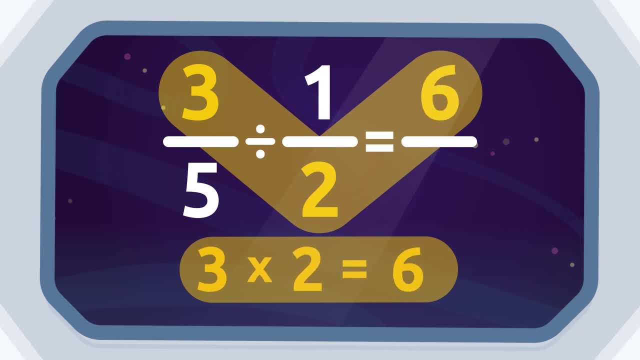 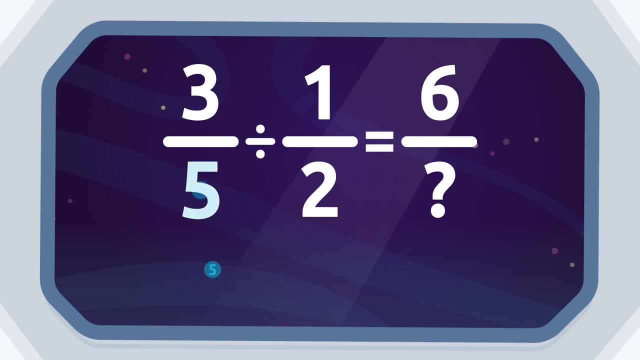 Meaning 3 by 2, which equals 6. the numerator of the product is 6. Now to find the denominator of the product, we multiply the denominator of the first fraction by the numerator of the second fraction, Meaning 5 by 1, which equals 5. the denominator of the product is 5. 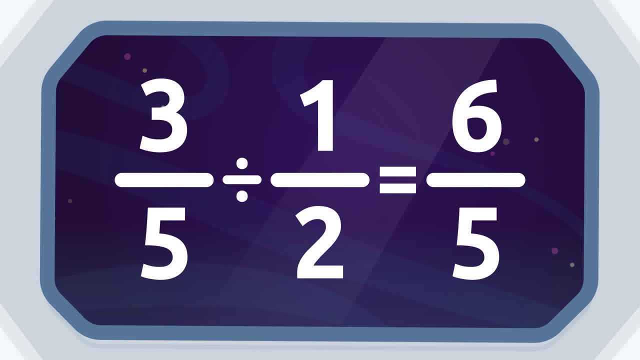 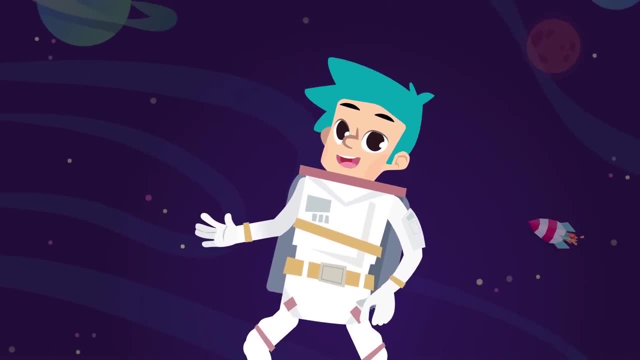 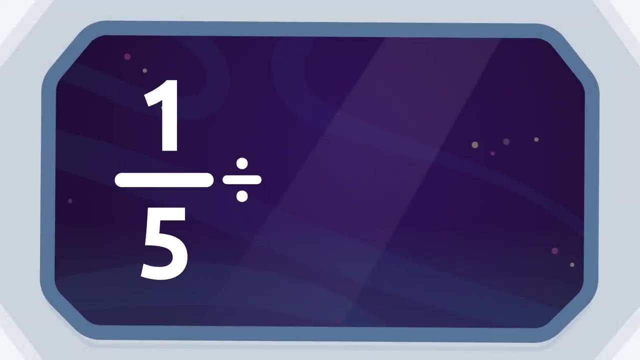 So 3 fifths divided by 1 half equals 6 fifths. Excellent, Let's look at the next example. would you like to try doing this one yourself? 1 fifth divided by 1 third equals 3 fifths. Let's find out if you got it right. 1 fifth divided by 1 third equals 3 fifths.